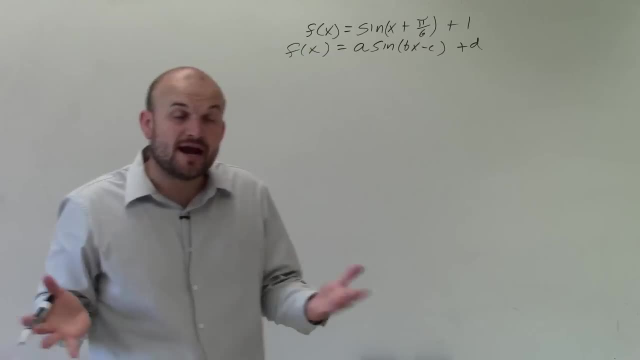 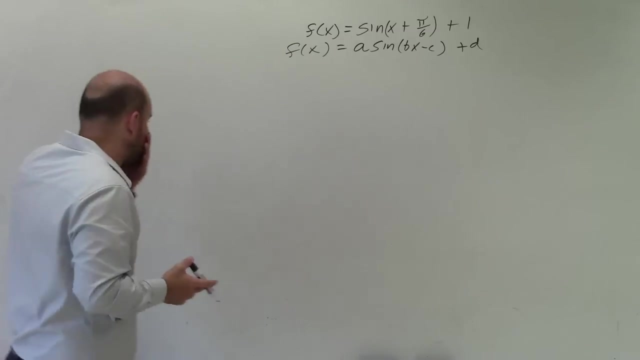 a, d. So how are those values going to affect our parent graph? Because we need to kind of understand at least what the parent graph looks like and then go ahead and apply that to our different transformations. So what we want to do to solve for sine, we want to. 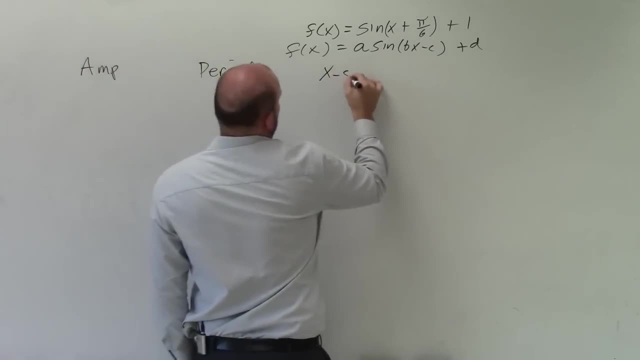 figure out the amplitude, the period, the x scale, the phase shift And the vertical transformations. So I'm going to kind of go through how we figure out each one of those. The amplitude is the absolute value of a. The period is 2 pi divided by. 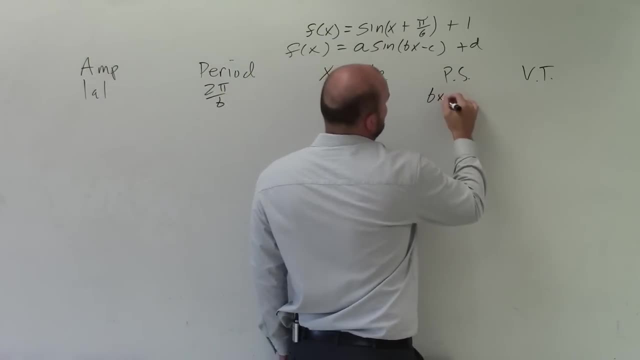 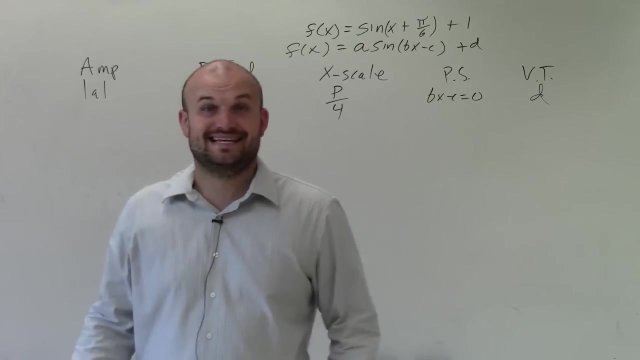 b. X scale is the period divided by 4.. Phase shift is bx minus c, equal to 0. Whatever is inside your parentheses set equal to 0. And your vertical transformation is d. Did I say that all fast enough? Sorry, I've just made a couple of these videos, so it's the same. 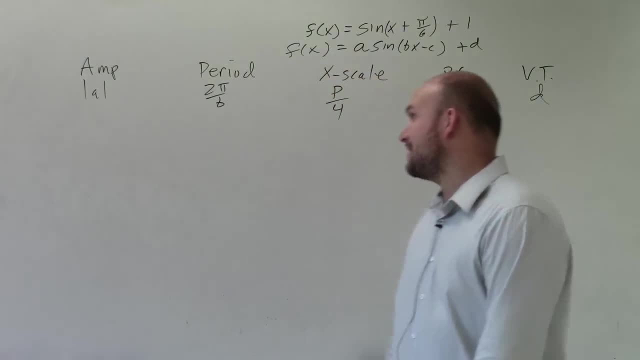 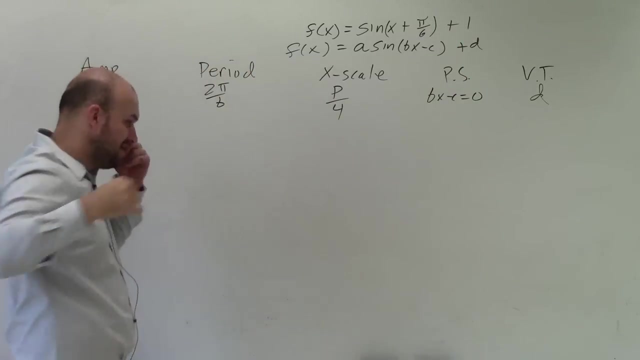 thing over and, over and over again. So I kind of go a little quick. All right, So we can look in this equation. So now we're going to be looking up here and seeing what do we have and how is it going to affect our graph? So our amplitude is our. 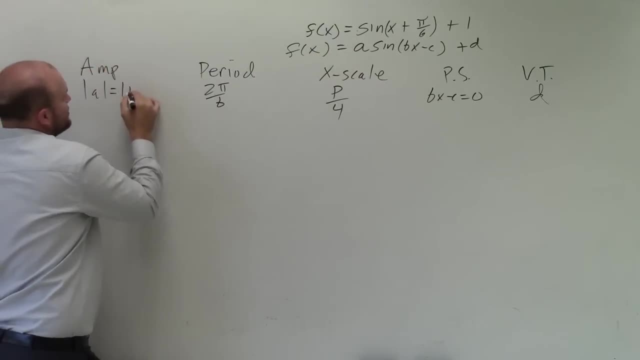 a. Well, we don't have an a. Well, technically we do, It's a 1.. So the absolute value of 1 is just 1.. Our period is going to be 2 pi divided by b, which in this case again is: 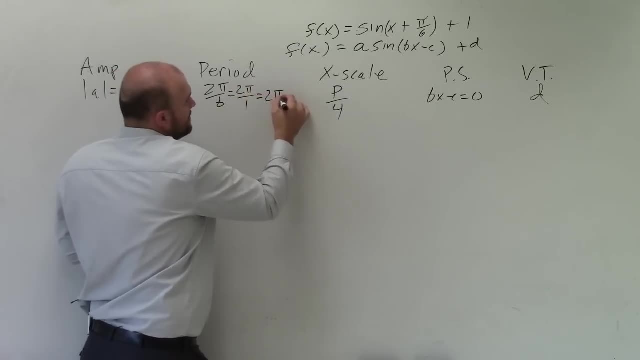 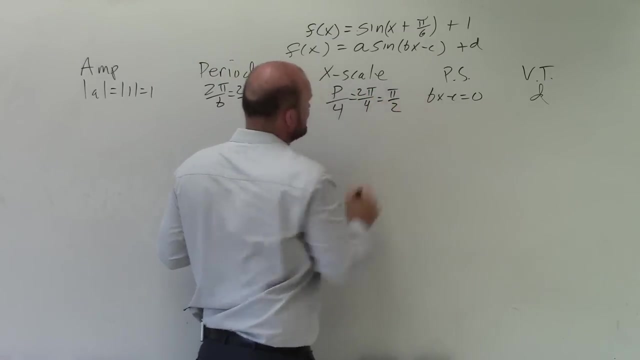 1.. So 2 pi divided by 1 is just 2 pi. Our x scale is our period divided by 4.. So I take 2 pi divided by 4, which equals pi halves, And so far this is all the same as our parent graph. However, now we're getting something. 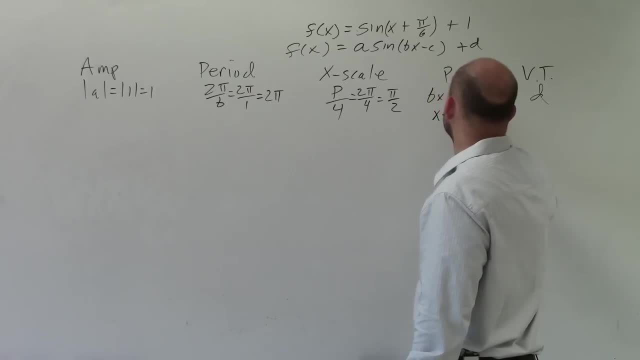 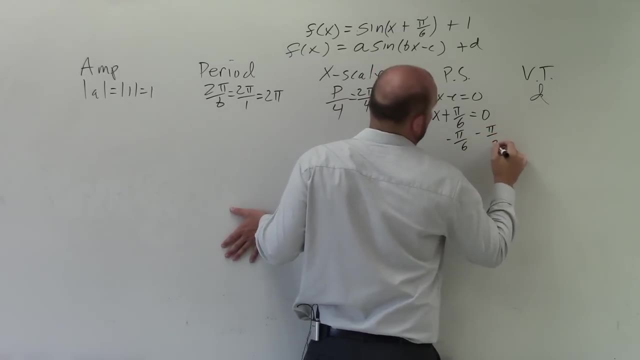 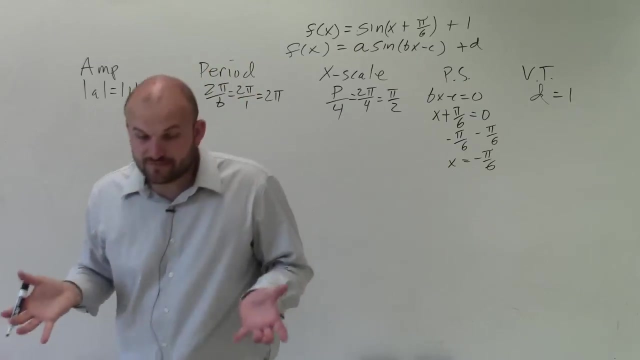 a little bit different with our phase shift, which is x plus pi over 6 equals 0. So to solve for x I need to subtract pi over 6. Subtract pi over 6.. x equals a negative pi over 6. And my vertical translation is equal to 1.. That means I'm going to actually take 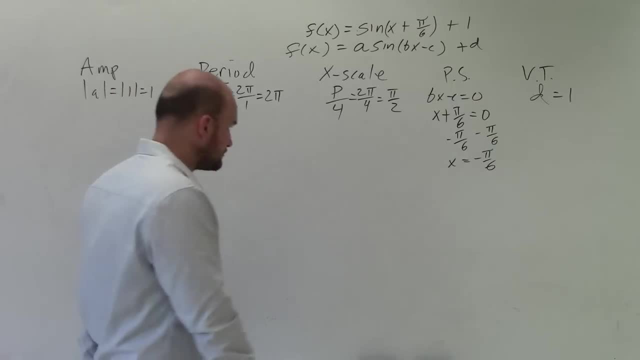 the whole graph and shift it up 1.. Now, All right. So what I'm going to do is I am going to graph each one of these translations separately, to kind of combine them all together. So I'm going to do one at a time. Now the first. 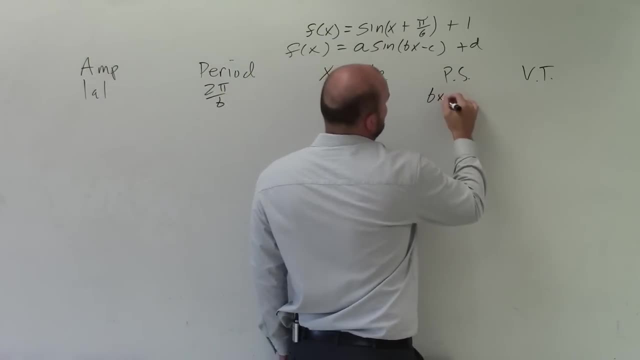 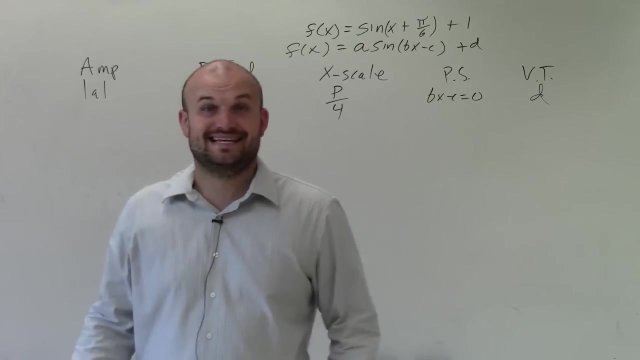 b. X scale is the period divided by 4.. Phase shift is bx minus c, equal to 0. Whatever is inside your parentheses set equal to 0. And your vertical transformation is d. Did I say that all fast enough? Sorry, I've just made a couple of these videos, so it's the same. 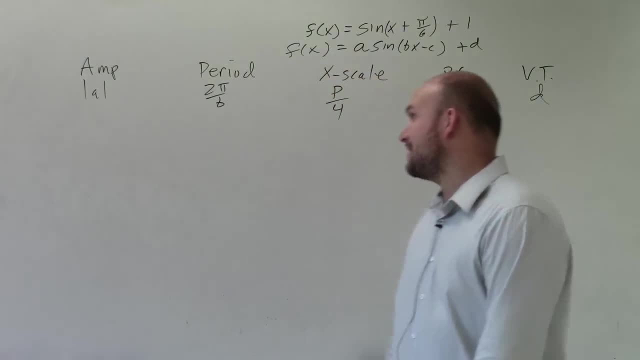 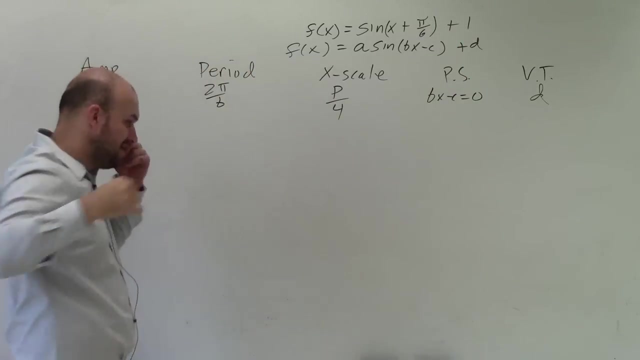 thing over and, over and over again. So I kind of go a little quick. All right, So we can look in this equation. So now we're going to be looking up here and seeing what do we have and how is it going to affect our graph? So our amplitude is our. 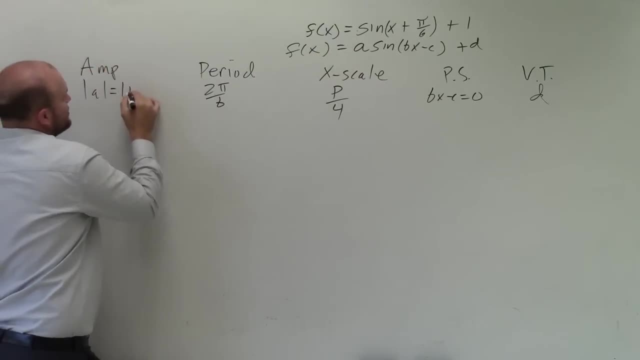 a. Well, we don't have an a. Well, technically we do, It's a 1.. So the absolute value of 1 is just 1.. Our period is going to be 2 pi divided by b, which in this case again is: 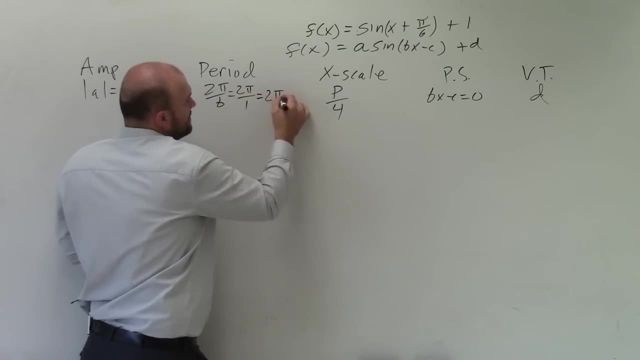 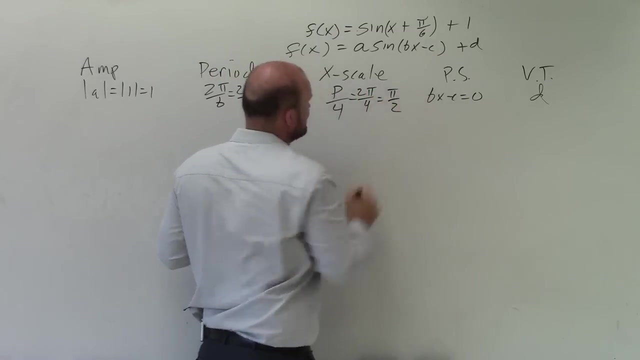 1.. So 2 pi divided by 1 is just 2 pi. Our x scale is our period divided by 4.. So I take 2 pi divided by 4, which equals pi halves, And so far this is all the same as our parent graph. However, now we're getting something. 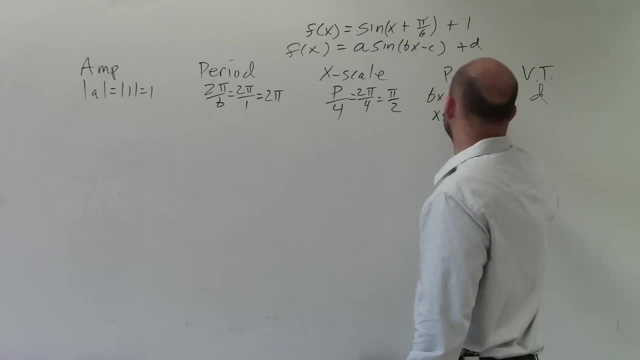 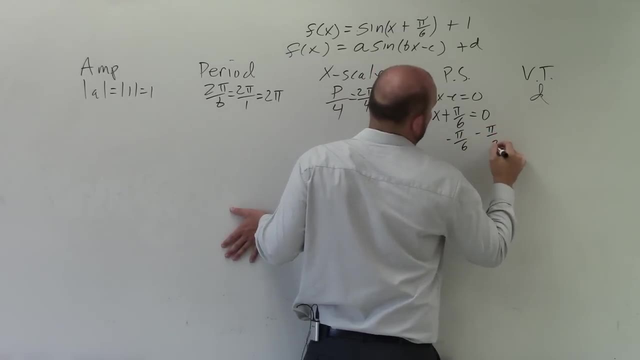 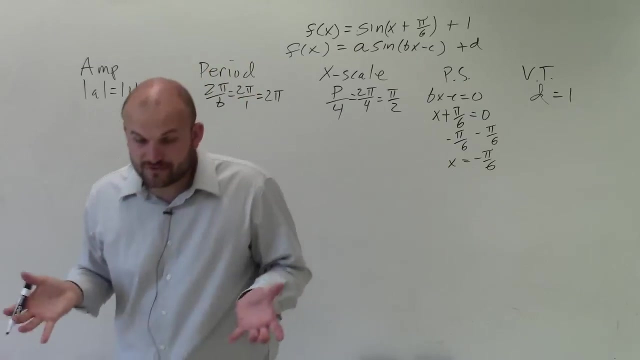 a little bit different with our phase shift, which is x plus pi over 6 equals 0. So to solve for x I need to subtract pi over 6. Subtract pi over 6.. x equals a negative pi over 6. And my vertical translation is equal to 1.. That means I'm going to actually take 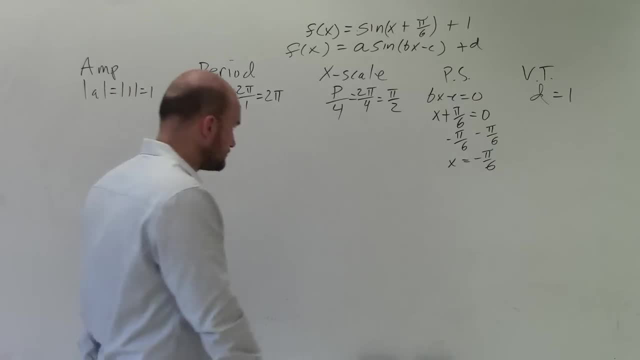 the whole graph and shift it up 1.. Now, All right. So what I'm going to do is I am going to graph each one of these translations separately, to kind of combine them all together. So I'm going to do one at a time. Now the first. 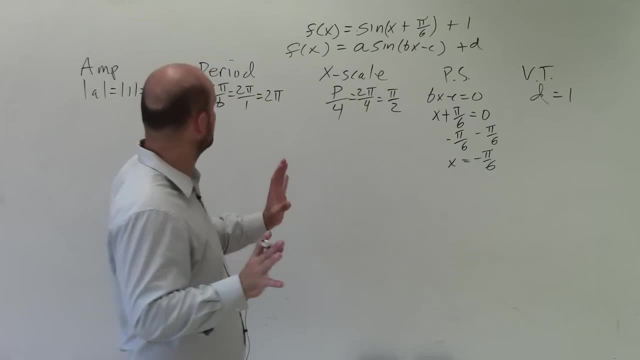 thing we want to do is make sure we understand what actually never mind, Never mind, I'm just going to do. I'm actually going to start it correctly because I don't want to mess up this phase shift. This is going to be not so fun. 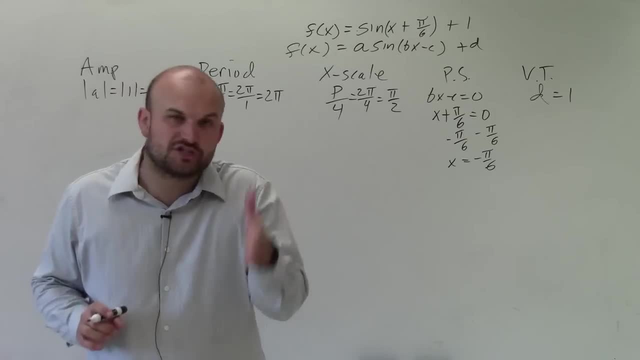 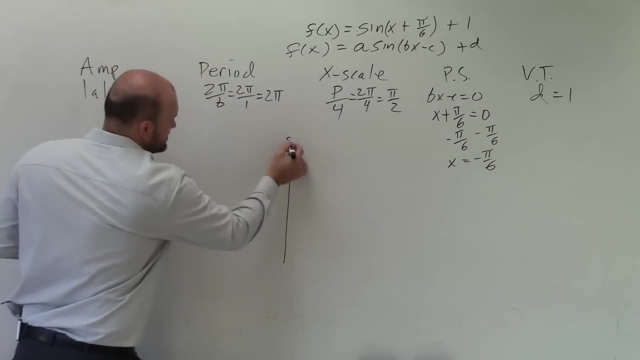 So what I typically like to do: when we graph the sine graph, we always kind of start at 0, right, That's what we call the initial period. But when we have a phase shift, I want to start at my phase shift. So let's pretend here is 0.. OK, And let's start at. 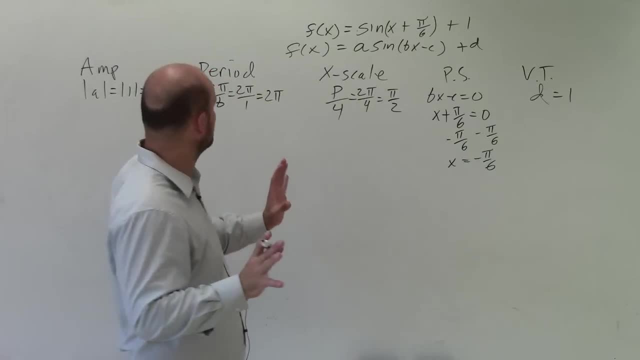 thing we want to do is make sure we understand what actually never mind, Never mind, I'm just going to do. I'm actually going to start it correctly because I don't want to mess up this phase shift. This is going to be not so fun. 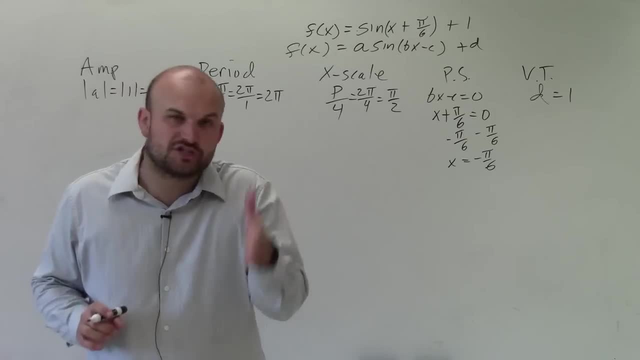 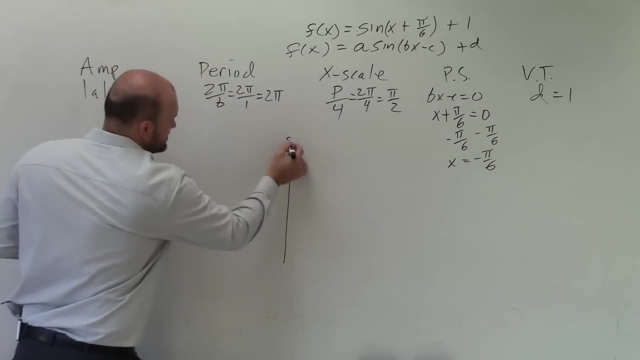 So what I typically like to do: when we graph the sine graph, we always kind of start at 0, right, That's what we call the initial period. But when we have a phase shift, I want to start at my phase shift. So let's pretend here is 0.. OK, And let's start at. 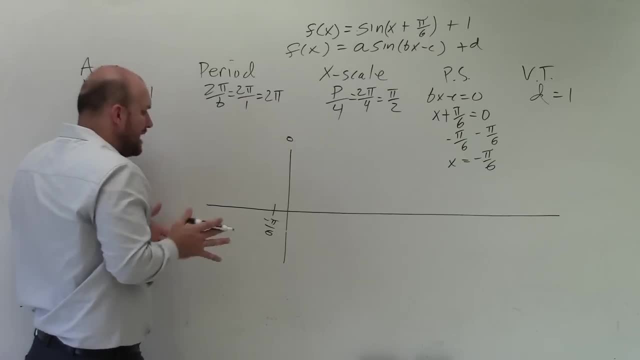 negative pi over 6.. Now 0 usually was our starting point, But now negative pi over 6 is going to be. But remember, for our period there are four x scales, So I have 1,, 2,, 3,. 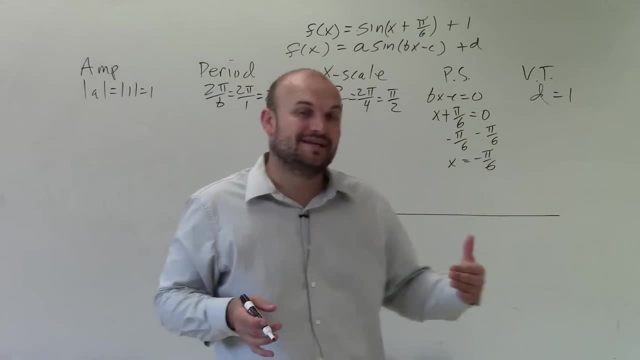 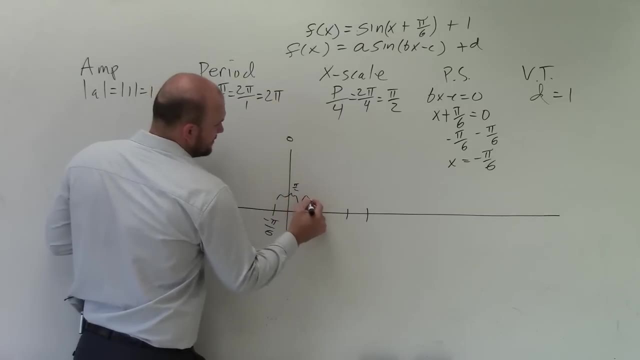 4. Now we just need to determine what are each one of those. Now we know. the distance between each one of those is pi halves, right? That's pi halves. That's pi halves. The distance to this one is pi halves. These two are pi halves, So the distance between each one of 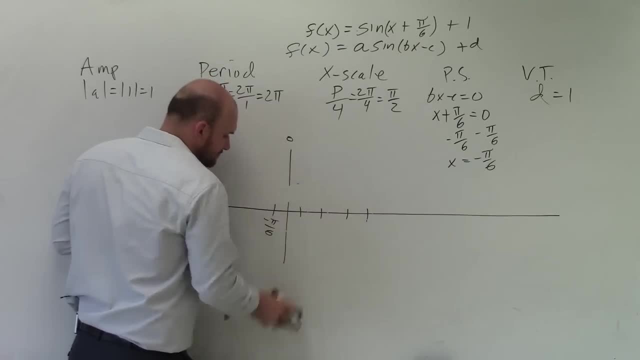 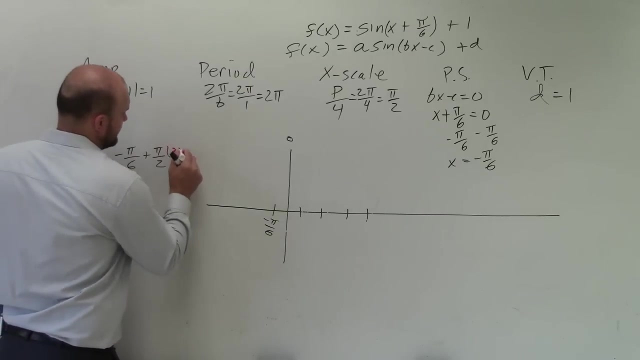 these is all pi halves. We just now need to be able to figure out what exactly the value. So to do that, just take negative pi over 6 plus pi over 6.. Now we've got well, those are pi halves We need to. 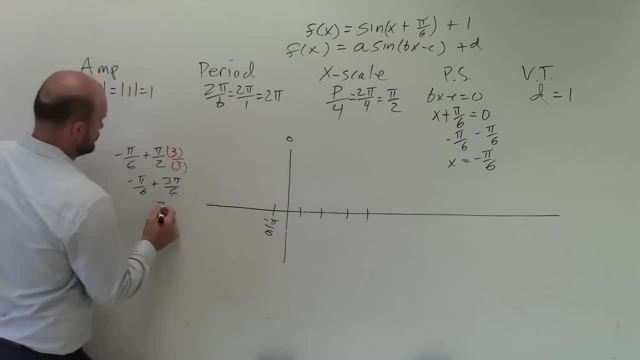 knows what that's equal to in terms of both x squared and pi. true, That's two pi over 6.. I'm going to get that by 2 pi over 6 have 3 pi over 6.. That's 2 pi over 6.. 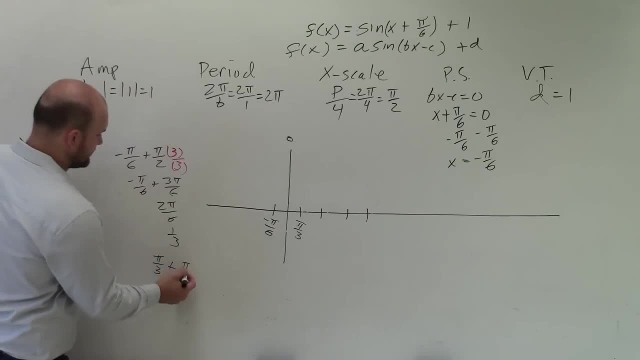 plus pi halves. Well, let's do 2 pi over 6.. 2 pi over 6 plus pi halves. Again, multiply by 3 over 3. And therefore you get 5 pi over 6.. So then this would be: 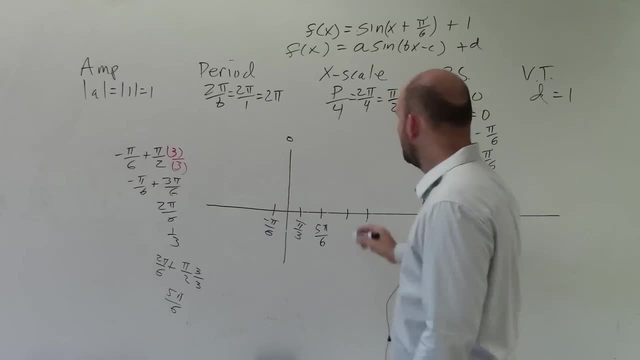 5 pi over 6.. The next one is going to be 8 pi over 6.. If you kind of just follow the pattern, this is 2 pi over 6, 5 pi over 6,, 8 pi over 6,. 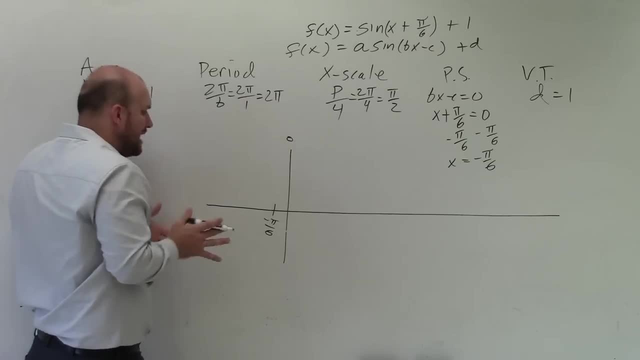 negative pi over 6.. Now 0 usually was our starting point, But now negative pi over 6 is going to be. But remember, for our period there are four x scales, So I have 1,, 2,, 3,. 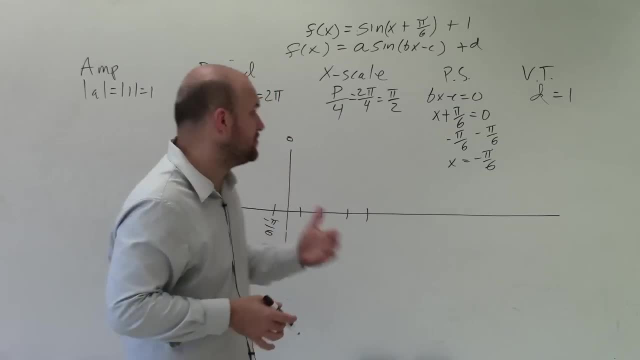 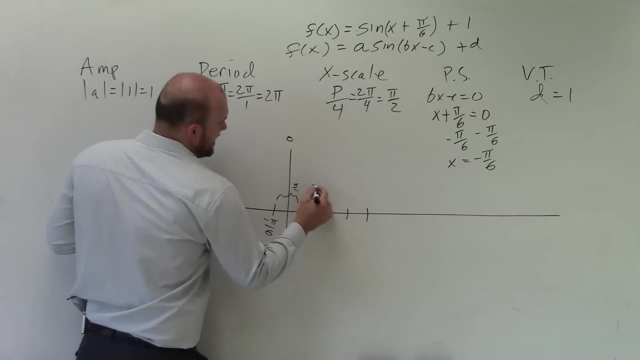 4. Now we just need to determine what are each one of those. Now we know. the distance between each one of those is pi halves, right? That's pi halves. That's pi halves. The distance to this one is pi halves. These two are pi halves, So the distance between each one of 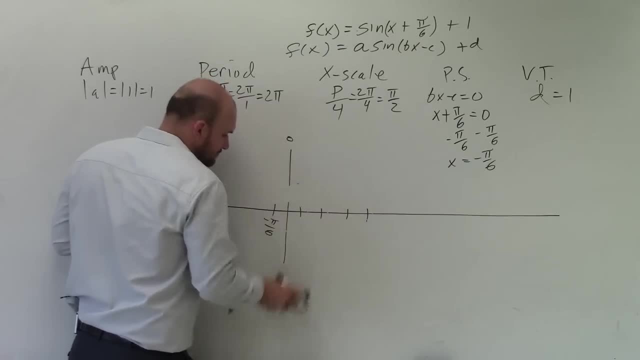 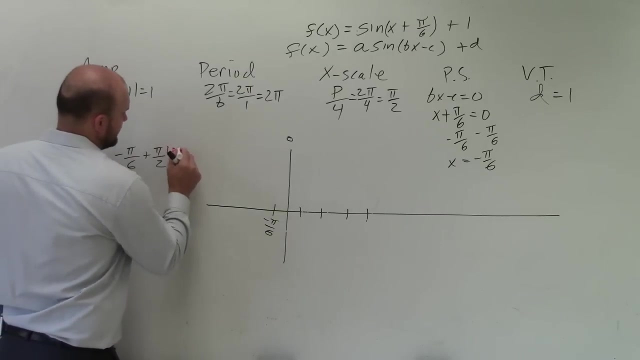 these is all pi halves. We just now need to be able to figure out what exactly the value. So to do that, just take negative pi over 6 plus pi halves. Well, to get that I need to get common denominators. I'm just doing a little fraction work And 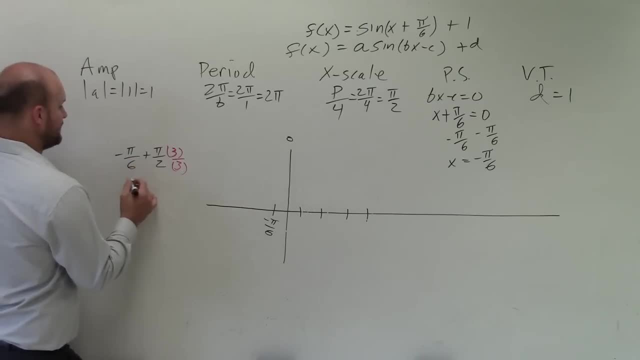 I'll show you how this is going to help me out as well. So therefore, I have negative pi over 6 plus 3 pi over 6,, which equals 2 pi over 6,, which equals 1 third. So this is. 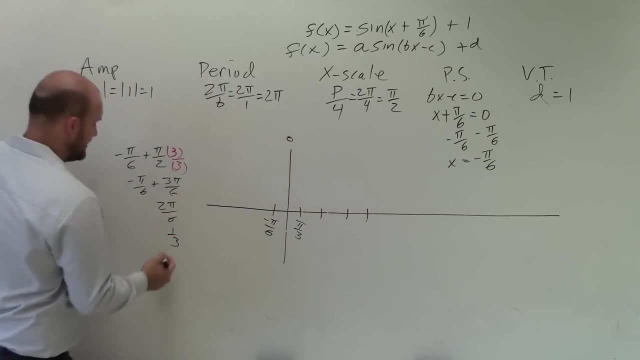 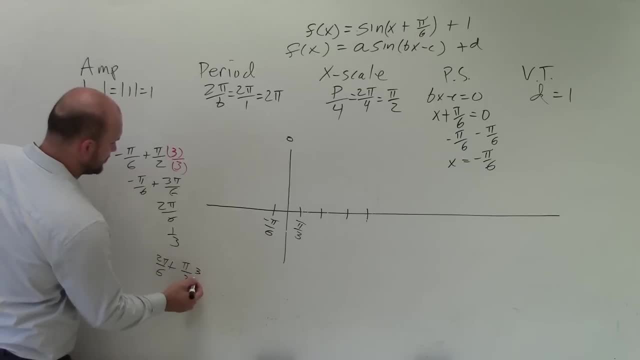 2 pi over 6, plus pi halves Again, multiply by 3 over 3. And therefore you get 5 pi over 6.. So then this would be 5 pi over 6.. The next one is going to be 8 pi. 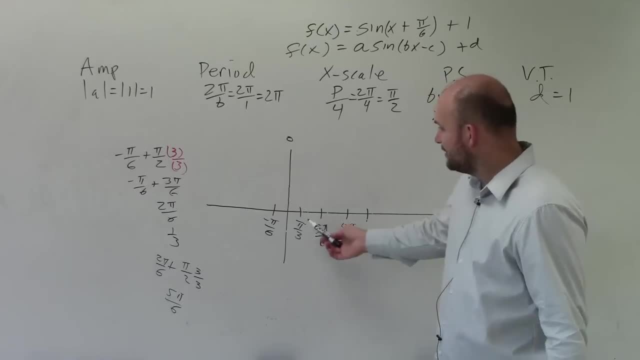 over 6.. If you kind of just follow the pattern, this is 2 pi over 6,, 5 pi over 6,, 8 pi over 6.. And this one would be 11 pi over 6.. And then let's do 2 periods. The next one is going to be: 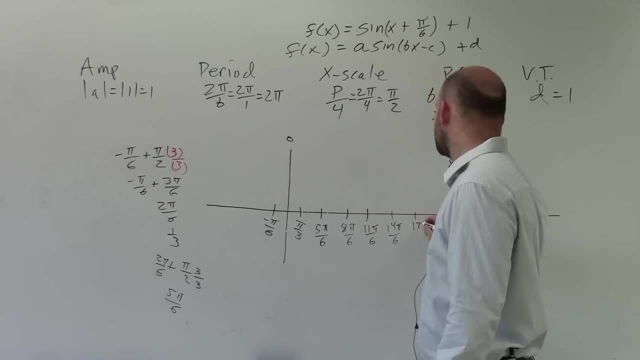 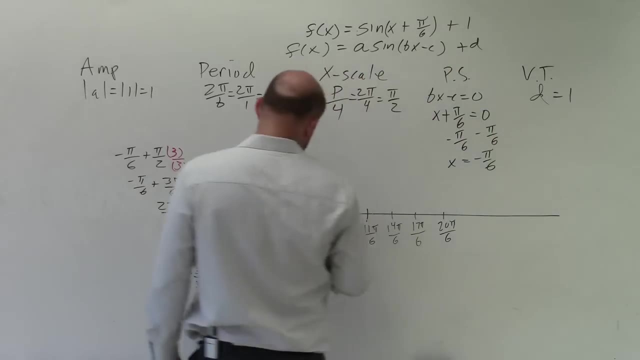 14 pie over 6.. 17 pi over 6.. 20 pi over 6.. So let's see, you have 1,, 2, 3, 4,, 1,, 2,, 3, and then we do one more. 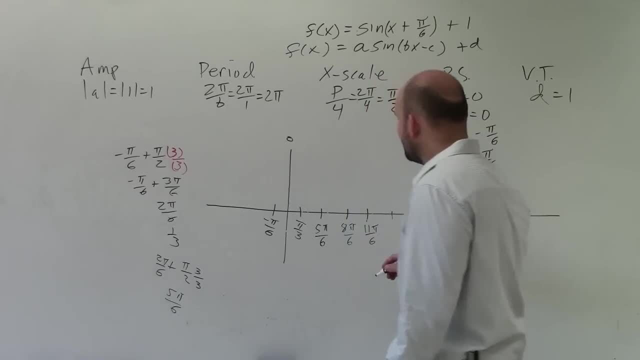 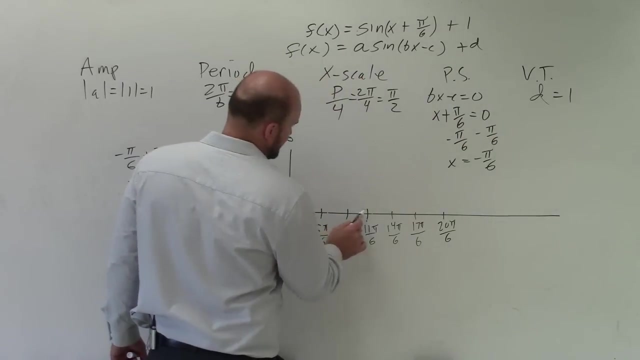 and this would be 11 pi over 6.. And then let's do two periods. So the next one is going to be 14 pi over 6,, 17 pi over 6,, 20 pi over 6.. So let's see I have 1,, 2,, 3,, 4,. 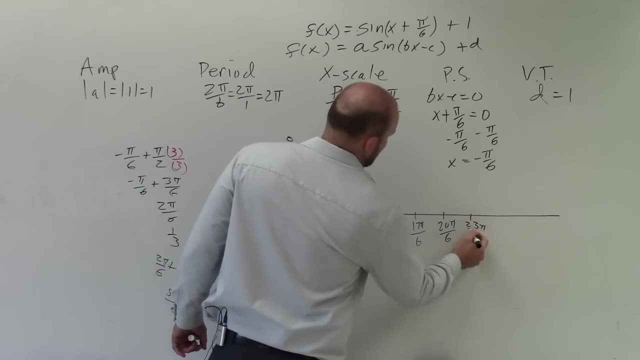 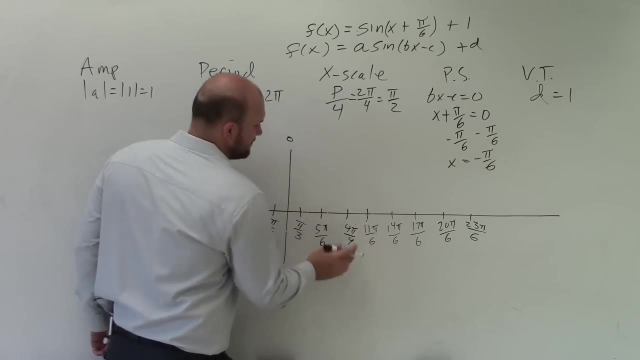 1,, 2,, 3, and then we do one more: 23 pi over 6.. Now obviously some of these we can reduce right, This can reduce down to 4 thirds: 4 pi over 3. This can be reduced down to 7 thirds. 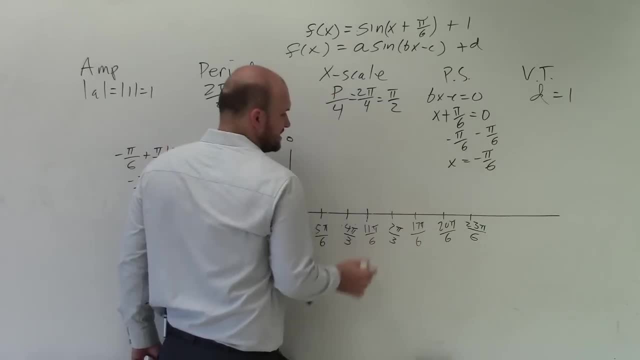 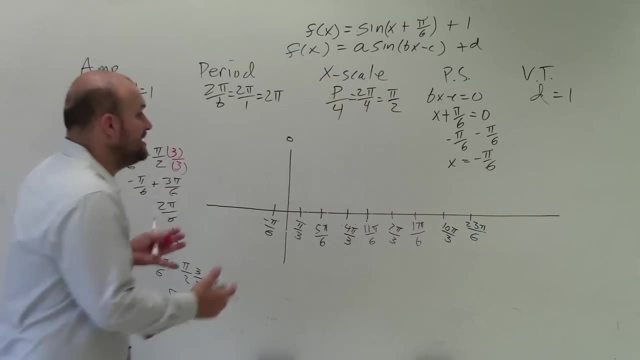 This can be reduced down to 10 thirds, Okay, So you can go ahead and reduce those. So now you have your x-scale, which I said. that's why I didn't want to graph the parent function in there, because I knew it was going to be a. 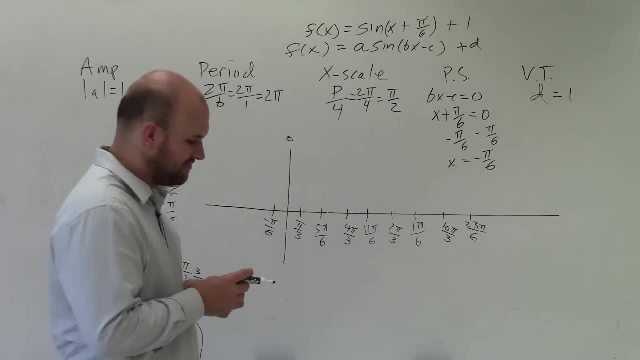 little difficult, Not really difficult. it's just going to kind of be a little confusing if we have the regular x-scale in there. So now we have our x-scale and we have our period, So 1,, 2,, 3, 4.. 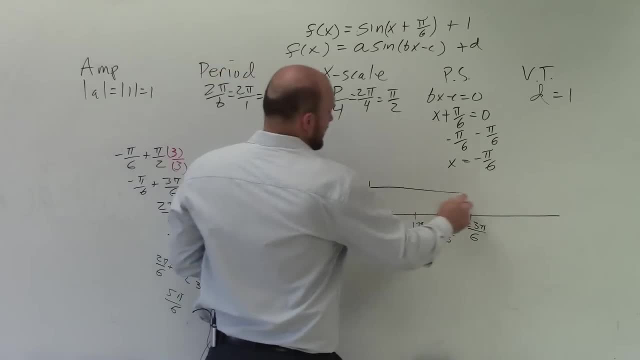 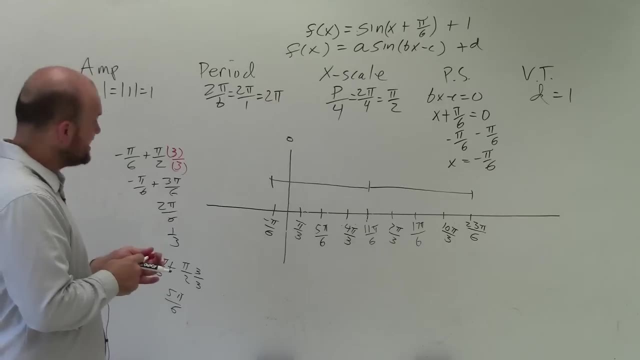 That's the period of my first, that's the first initial period and that's my second period. Usually we want to do at least complete two periods for our graph, Alright. so the last thing is, we know our amplitude goes up one and down one right. So even though we're still starting, remember that sine always starts at the. 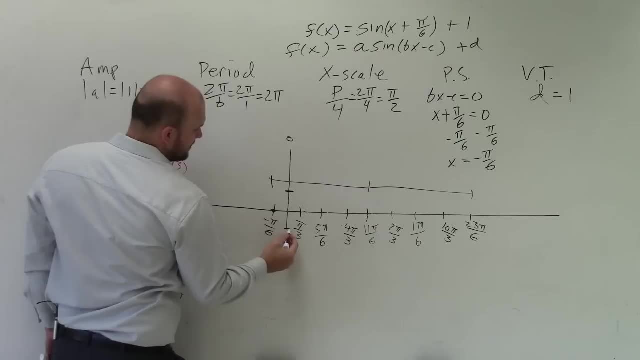 x-intercept and goes up to its maximum. So the maximum is 1 to negative 1.. But now what I'm doing? I just want to go on with my example. So yeah, usually I go up one to its max, to its to its intercept, to its minimum. 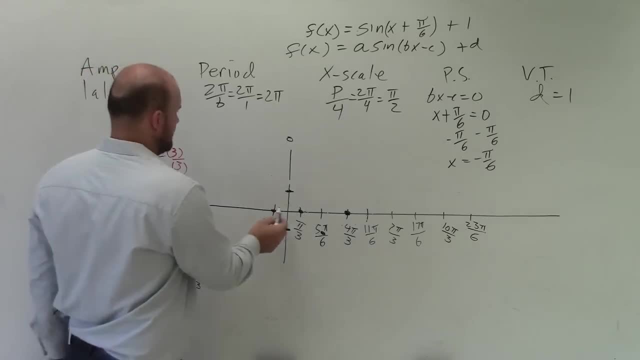 back up again. right, That is me satisfying. wait, why did I go? Oh, what am I doing? That's the next part, right Up here, down to its intercept, down to its minimum, back up. My apologies, I got confused with that x-intercept and that happens. 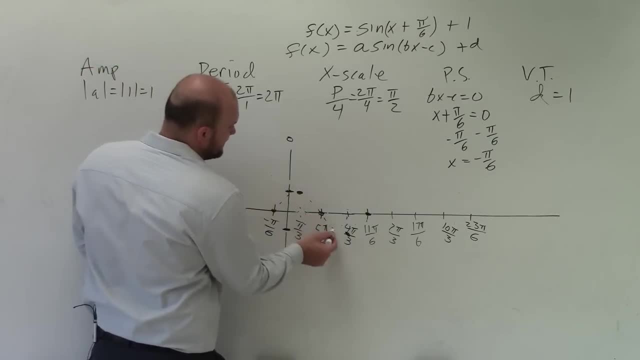 to a lot of students as well, So be careful. But now what I'm simply doing is taking each one, and so, instead of graphing this, this as my graph, I'm taking this and shifting it exactly one whole unit up. So what I like. 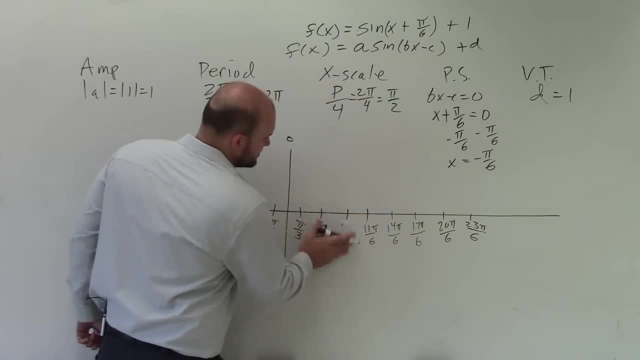 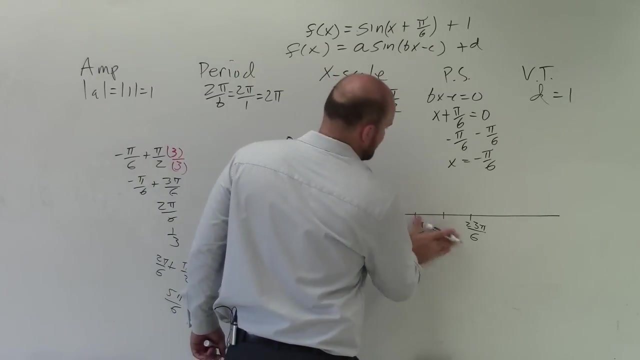 23 pi over 6.. Now, obviously some of these reconduce Right. This can reduce down to 4 thirds. 3, this can be reduced down to 7 thirds. This can be reduced down to 10 thirds. So you can. 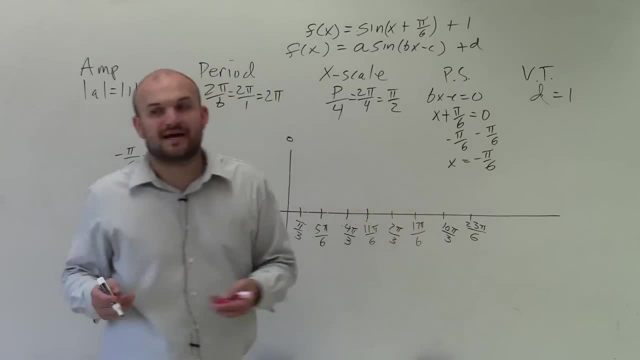 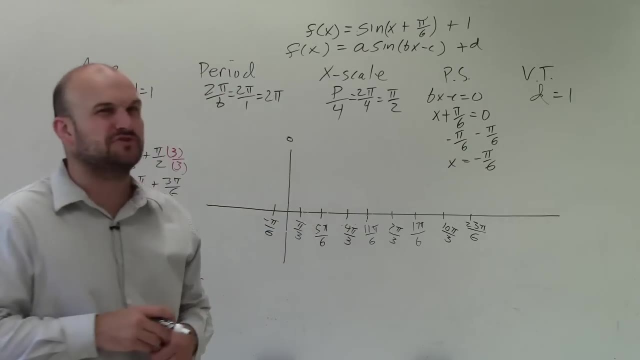 go ahead and reduce those. So now you have your x scale, which I said. that's why I didn't want to graph the parent function in there, because I knew it was going to be a little difficult- Not really difficult, it's just going to kind of be a little confusing if 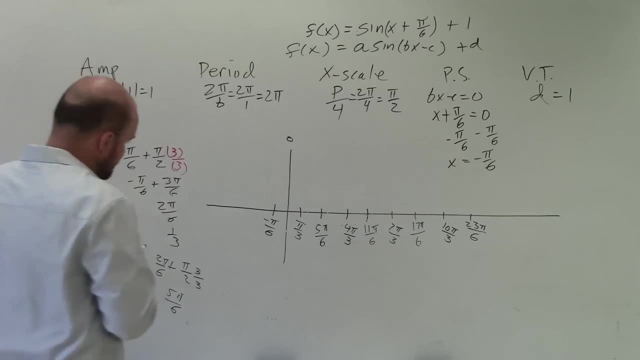 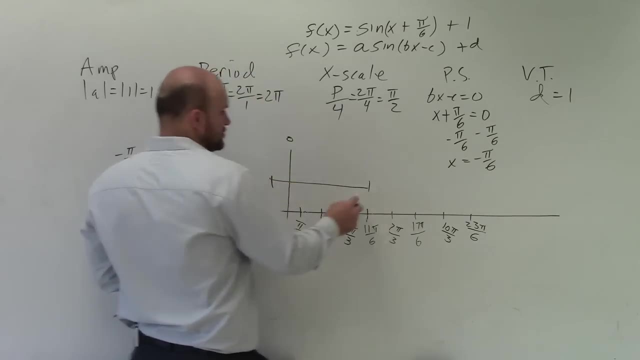 we have the regular x scale in there. So now we have our x scale and we have our period. So 1,, 2,, 3, 4, that's the period of my first, that's the first initial period and that's. 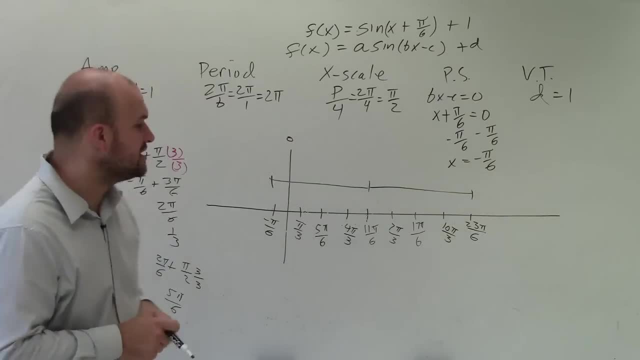 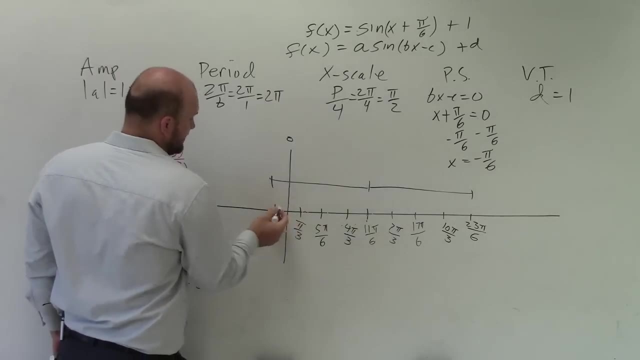 my second period, And usually we want to do at least complete two periods for our graph, Alright. so the last thing is, we know our amplitude goes up one and down one, right. So, even though we're still starting, remember that sine always starts at the x intercept. 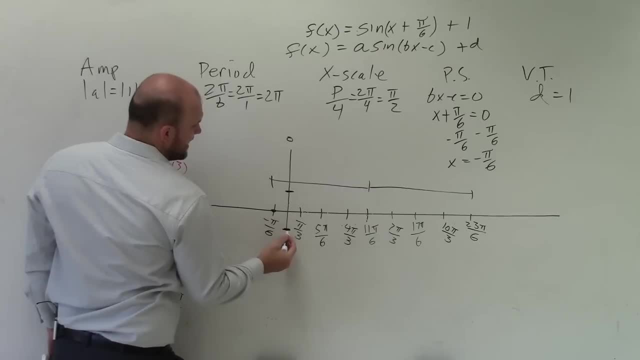 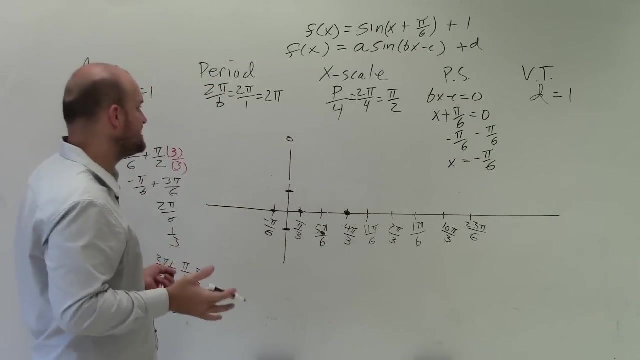 and goes up to its maximum. So the maximum is 1 to negative 1.. But now what I'm doing is: so, yeah, usually I go up one to its max, to its intercept, to its minimum, back up again. right, That is me satisfying. wait, why did I go? oh, what am I doing? That's. 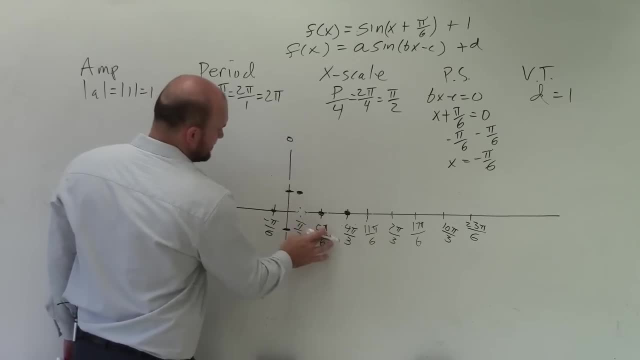 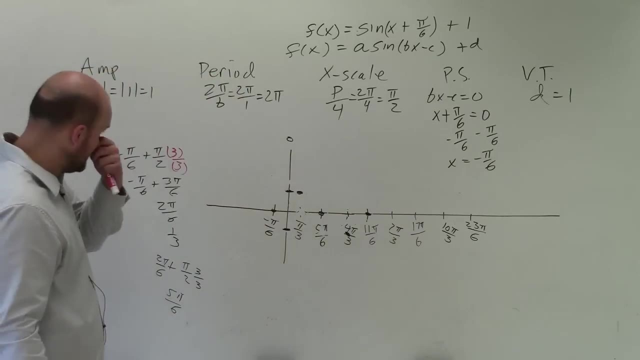 the next part, right Up here, down to its intercept, down to its minimum back up. My apologies, I got confused with that x intercept and it happens to a lot of students as well, so be careful. But now what I'm simply doing is taking. 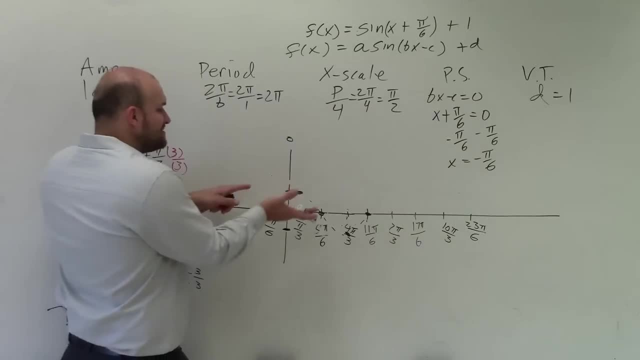 each one, and so, instead of graphing this as my graph, I'm taking this and shifting it exactly one whole unit up. So what I like to do a lot of times is, whenever I'm shifting up or down, I like to say: alright, where's the x-axis and how far am I moving it up? 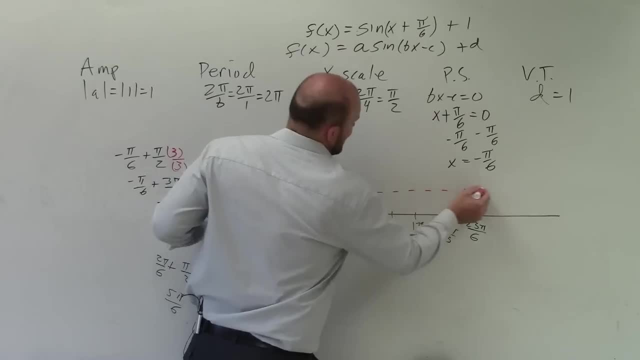 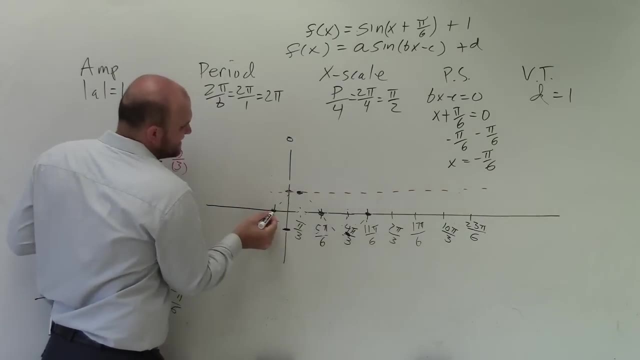 or down, Because if I'm moving it up I'm just going to rewrite that x-axis up above there. So now it makes a little bit more sense for me saying: oh well, this point was on the x-axis here, now it's on my moved up x-axis And then. so if that's one, I'm going. 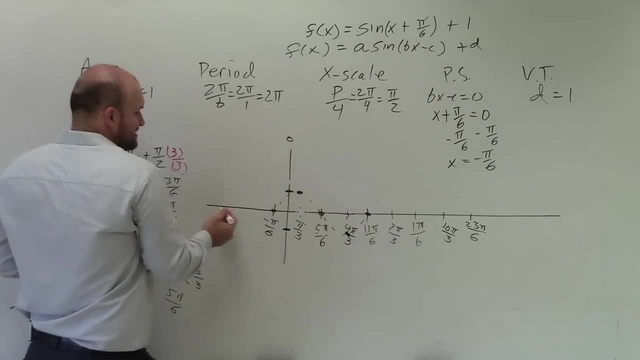 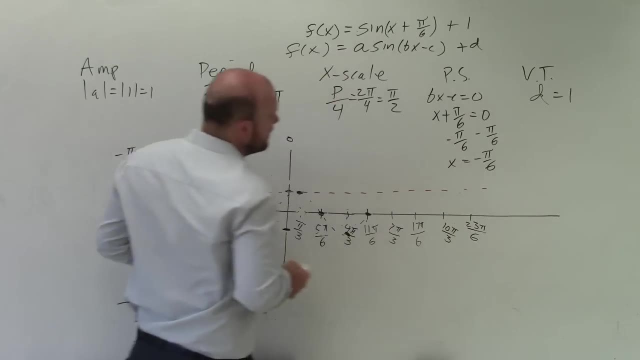 to do a lot of times is, whenever I'm shifting up or down, I like to say, all right, where's the x-axis and how far am I moving up or down? Because if I'm moving it up, I'm just going to rewrite that x-axis up above there. So now it makes a little bit more sense for me. 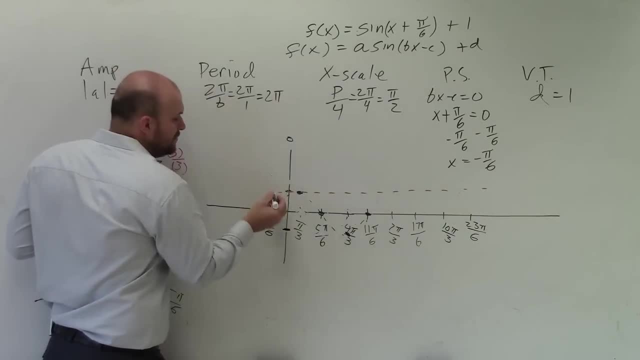 saying: oh well, this point was on the x-axis here, Now it's on my moved up x-axis And then so if that's one now I need to go up to two. So one up two. back to my imaginary 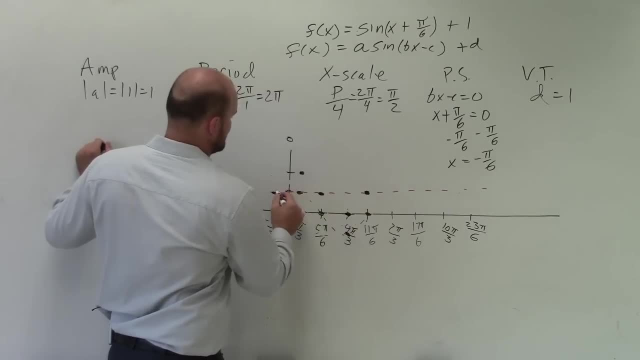 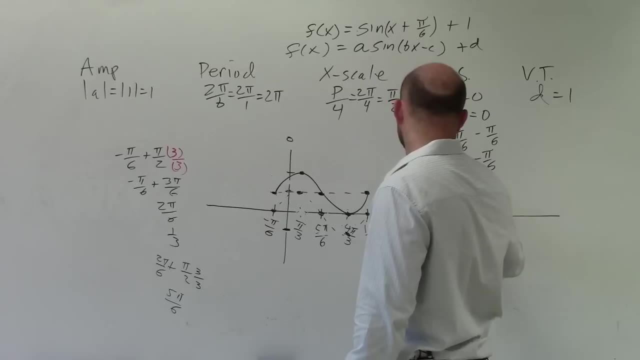 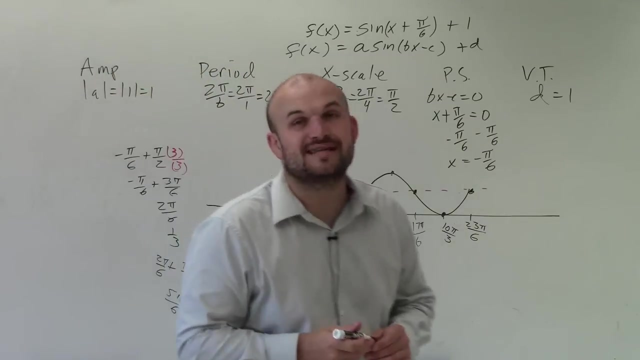 axis. now to its minimum, back up to the axis. So now you can see. my graph looks something like this, And then I will just continue the pattern up there. So again, obviously, ladies and gentlemen, this continues on and on forever, but that is at least your two initial periods. 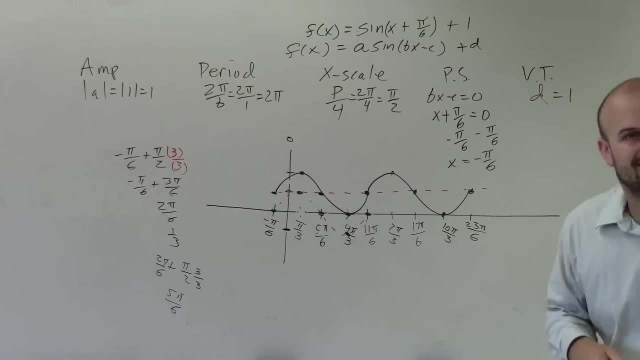 for how to graph sine Sine of x plus pi over 6 plus 1.. Thanks. 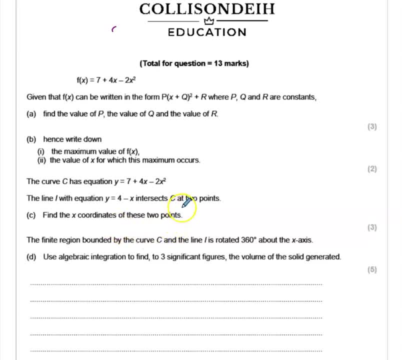 Hi, welcome to part 2 of my solution to this 13 mark examination question. In part 1, which you can see among my videos. it's entitled 13 mark question, part 1, we looked at solving the sections A and B, where the emphasis was on. 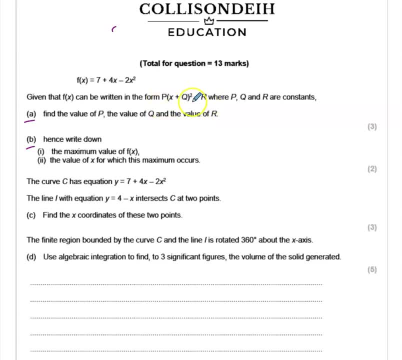 how to complete the square for any quadratic expression and also using a completed square to work out what our maximum maximum value and where it occurs, as far as the x-coordinate of that maximum point. and we were able to find that successfully. So with this question, now we're going to focus on